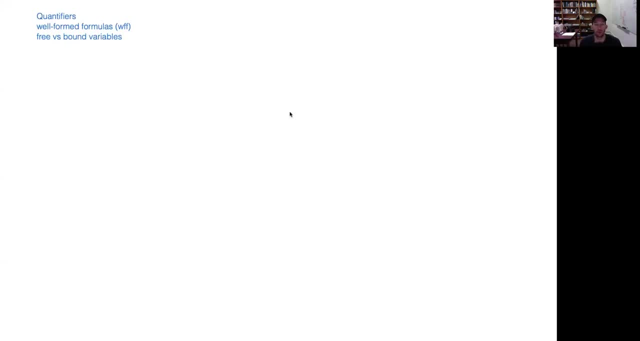 Welcome to the second lecture on quantifiers. In this video we're going to get into some more details about how quantifiers and variables work together. So the first thing we're going to talk about are, again, the two quantifiers that we're going to use: the universal and the existential. 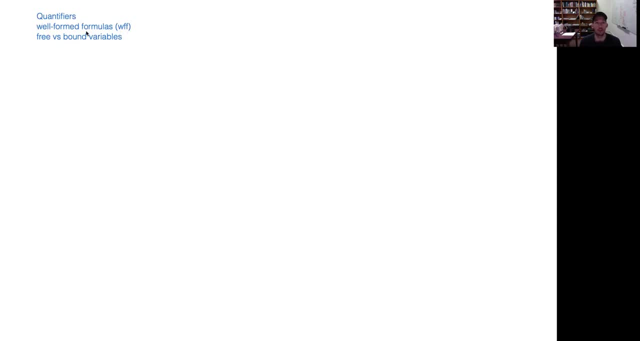 I'll briefly say something about well-formed formulas and then we'll talk about the distinction between free and bound variables. So remember, the idea behind a variable is that it works kind of like a name, in that it sits in an argument spot of a predicate. So if we have a 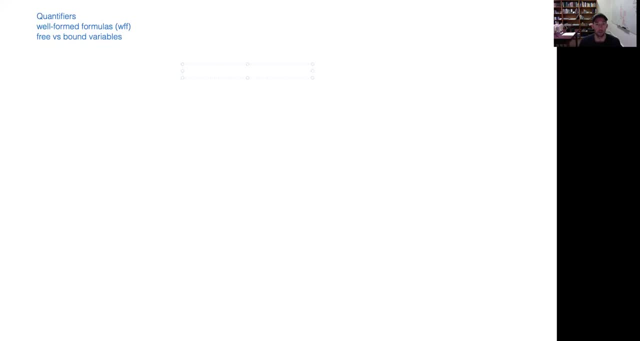 predicate. let's say sorry if we have a predicate like Tet and we had. we're looking in Tarski's world right. we're looking at Tarski's world right. we're looking at Tarski's world right. 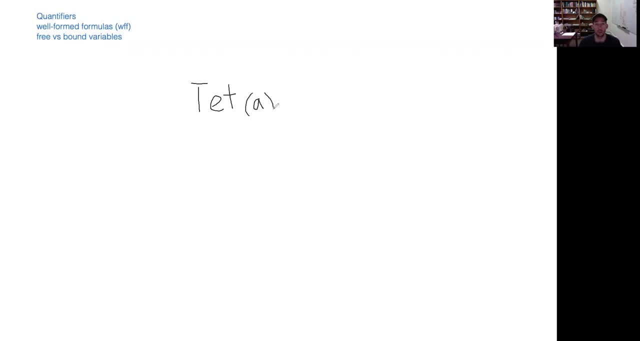 we could use something like a as as a name, but with variables. variables are kind of like names in that that sit in these argument spots, But instead but they're also totally unlike names and that they don't refer to a specific object. So that's one of the key features that distinguishes. 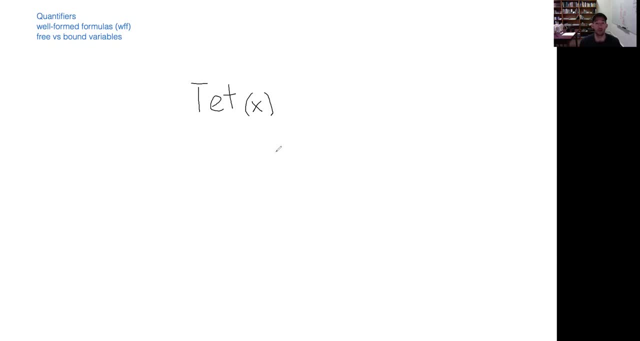 variables from names or constants. Names or constants refer to a specific object or a predicate, So we'll deal with all of those. now Let's copper, All right. so First of all, can I start at bi- 600 in three words. Okay, go wide a little, all right. So that's comes down to 1003 and 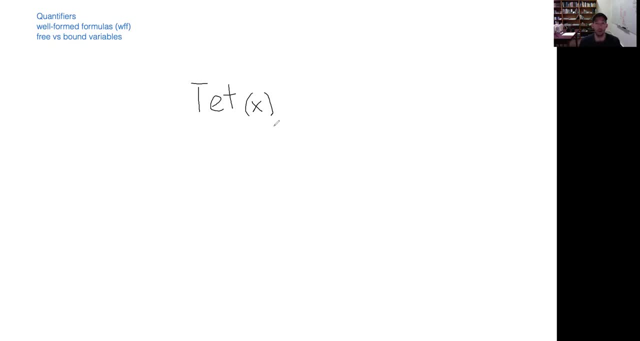 but variables will not Okay. so the basic idea behind a well-formed formula- or, as we'll sometimes write as a shorthand, WFF or WIF as it's sometimes known, is almost like a sentence, except that some of the names or constants. 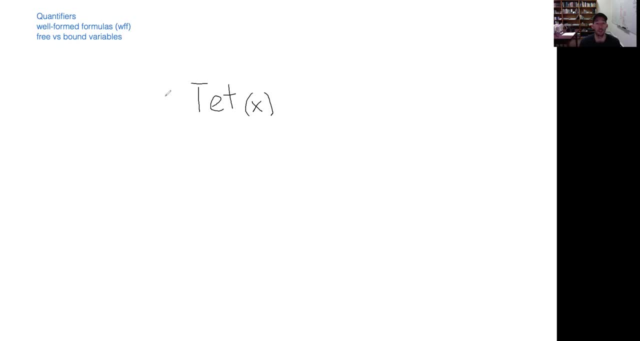 might have been replaced with a variable, but we don't yet see any particular type of quantifier, or there are what are called free instances of variables, like this X here. So if we think about variables as we've seen them in other contexts, right. 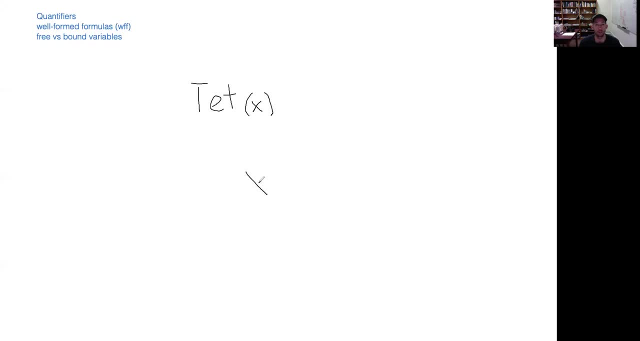 you might have like. in math you might have seen formulas that say something like: X plus X was equal to two X Here. right X doesn't name a particular number, right It can. you can plug in any type of number you like. 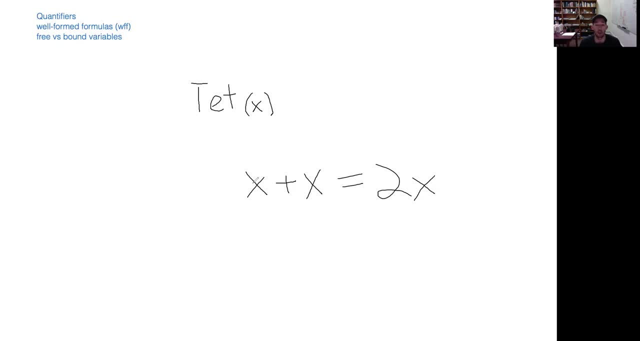 and then this equation will tell you about some relationship. So if X, for example, is refers to three or denotes three, then you know three plus three, that sum of that is going to be identical to if you took two and multiplied it by three, right? 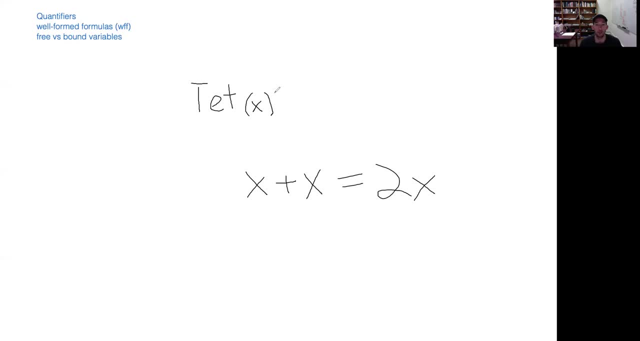 So in that case it would both be six. Same thing with the variables that we're going to use. in our language. X here can stand for any particular or can denote any object in the domain of discourse. So one of the things that's sort of implicit. 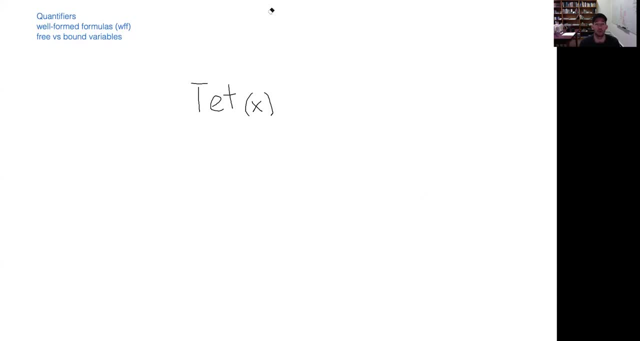 in mathematical uses of variables is that there's typically a universal quantifier implied, right? so for what I just had with that formula, the idea is that that formula holds for any number that you apply it to, So strictly speaking it would mean for any X. 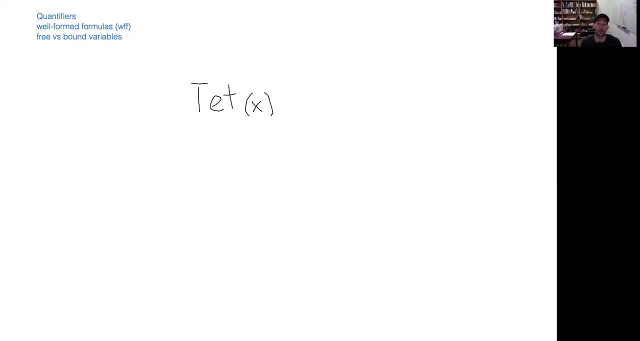 X plus X is equal to two X. There's an implicit universal quantifier there. Because we're going to have two different types of quantifiers in our language, we need to be clear about which particular quantifier we're using. So, for example, if I put out here the claim: 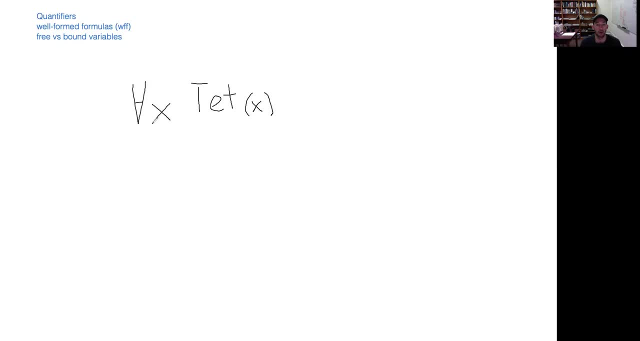 right, sorry, use a universal quantifier for all: x, tet, x. what this is saying is that everything in my domain, so everything in the Tarski world that you're looking at, is a tetrahedron. So this is. 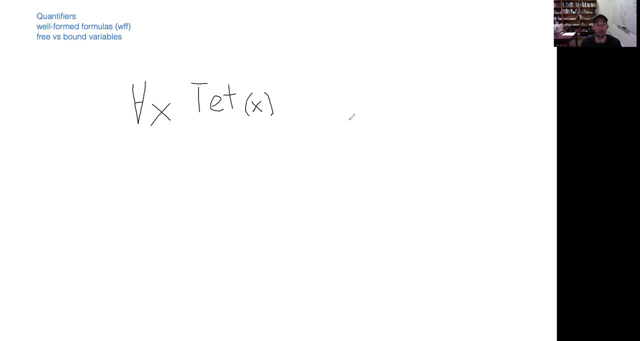 true, just in case, every object in Tarski's world is a tetrahedron and it's false if there's at least one object that is not a tetrahedron. Alternatively, instead of having the universal quantifier, we could have had instead the existential quantifier. and if we have the 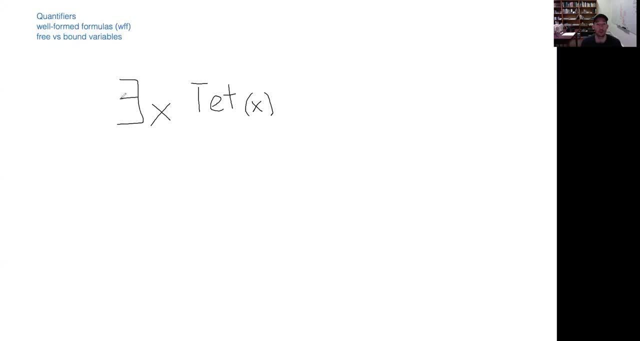 existential quantifier. this is now saying something different. This is now saying there is at least one object, right? there is some case- x, such that x is a tetrahedron. So this formula would now be true, just in case there is at least one object in the domain of discourse that is a. 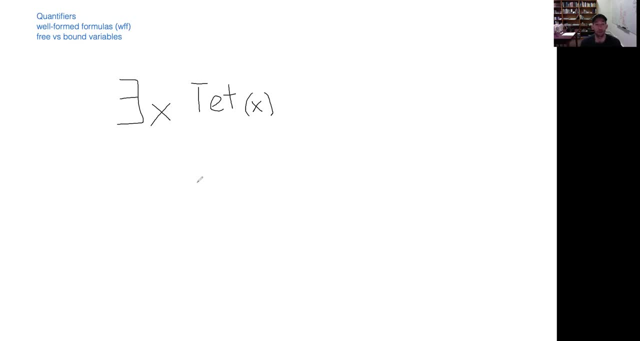 tetrahedron. So the difference between these, the three cases right. so the three cases is where we've got universal x, tet x and we've got the existential case right. there exists at least one x such that x. 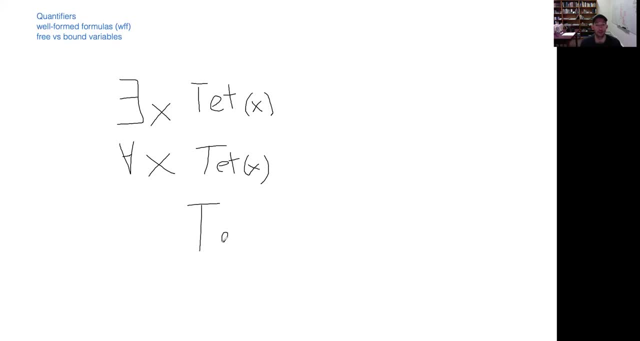 is a tetrahedron, and this third case just tet x. is that in these two? so in this formula, and in this formula we say the variable is bound. Oh dear, There we go. And here, in this case, the variable x. 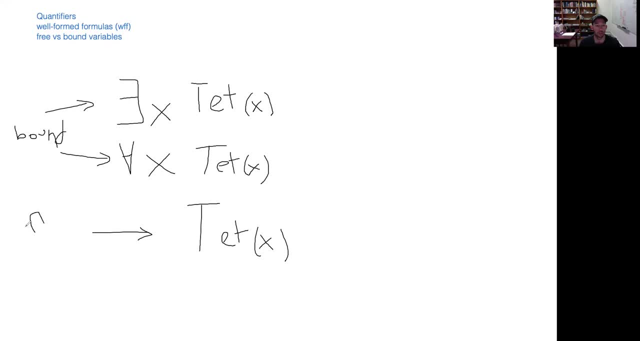 is free. So I should be clear: these arrows are not actually pointing to the quantifiers right. these arrows are actually pointing to this instance of the variable, right here. So here x is bound by this quantifier, The existential quantifier. 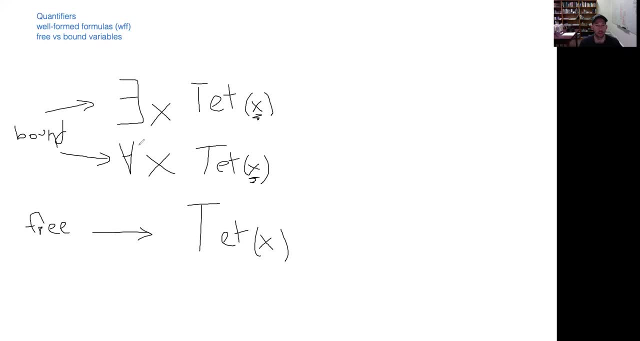 This instance of x is bound by this quantifier- quantifier right here- and this x in this formula is not bound by any quantifier at all. right, so we say instead that it is free, because it's we don't have a quantifier that tells us whether. 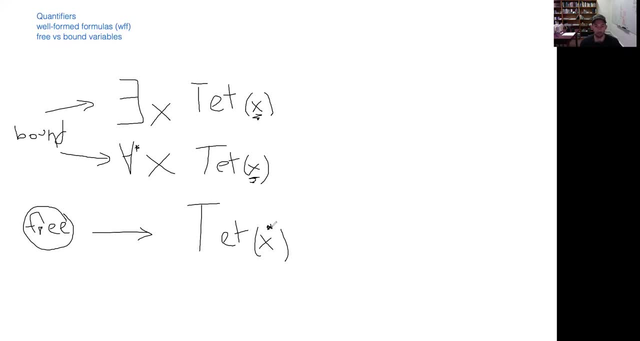 this x. this instance of this variable applies to just one particular instance, or at least one instance, or if it applies to all of them, okay. the reason why we make this distinction, in addition to being able to use two different quantifiers, is there might be multiple instances. 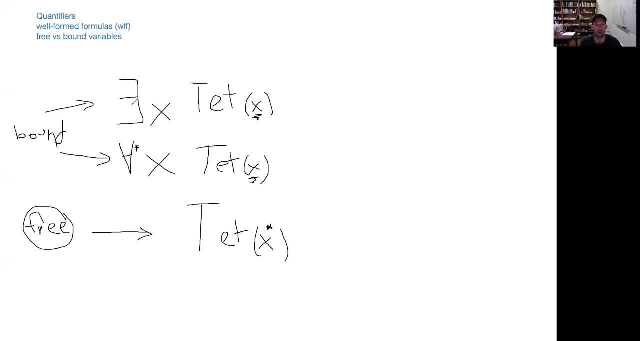 of some quantifier and it'll be important to distinguish which variable is being bound by which particular quantifier. so let me walk through an example here, make some space. let's know what i wanted to do. okay, so i want to consider two different sentences. let's see if i can. i think i can do this relatively. 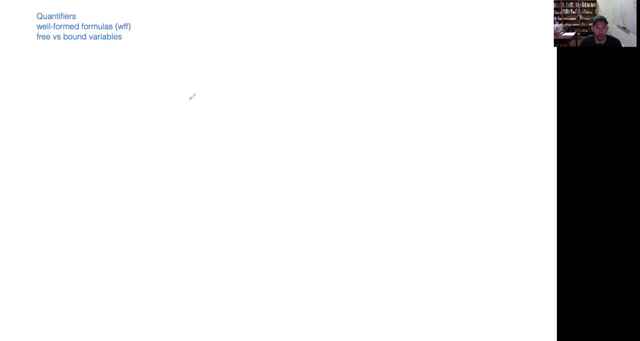 quickly. so let's consider the uh, the following sentence. so we're going to say: there exists an x, so there's at least one object that is a tetrahedron. so we have here now a quantified sentence, it's an existential sentence. there exists at least one tet and we might want to combine that now with a conjunction and say, okay, there exists. 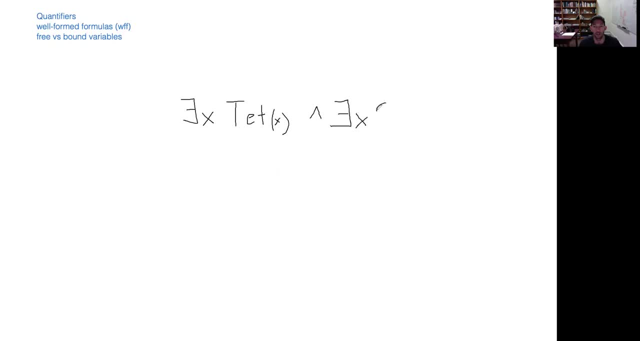 an x such that small x. So the thing to note is that this instance of x is being bound by that quantifier over there, and this instance of x is being bound by that quantifier there, and this sentence is ultimately a conjunction. It's conjoining. 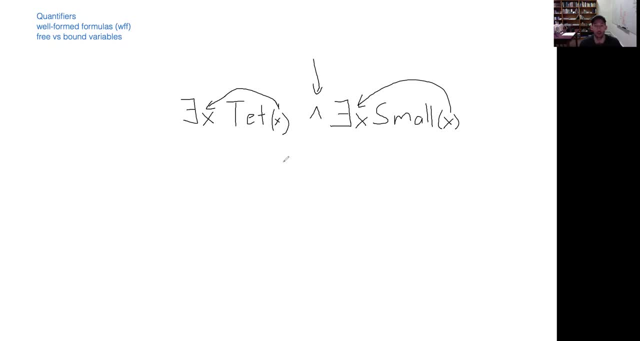 two different existential claims. So this sentence is true, just in case. there exists at least one tetrahedron and there exists at least one object that is small. So that would be satisfied in a world where you have, say, a large tetrahedron that is small. 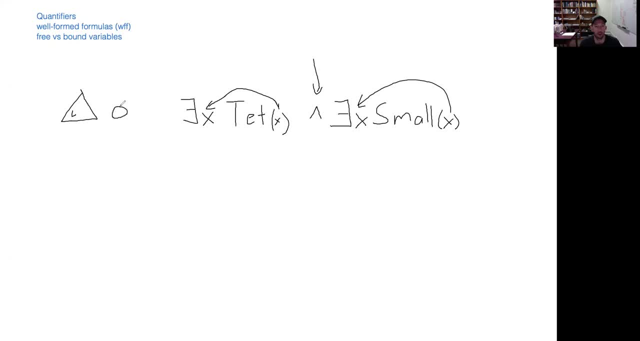 So this object is large and then you also have a small dodecagon. That's different than the following sentence, Suppose: instead of having the conjunction of two existential sentences, we said instead that there exists an x and we say x is a tet. 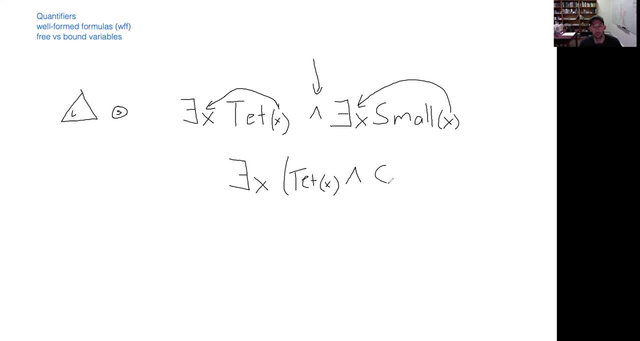 and we also have, is small institutional claim. So by that I mean that x, a total sum of this, and the last Connie from Winn, and x was small. Here the variable x, as you see it in two instances, is being bound by the same quantifier, that. 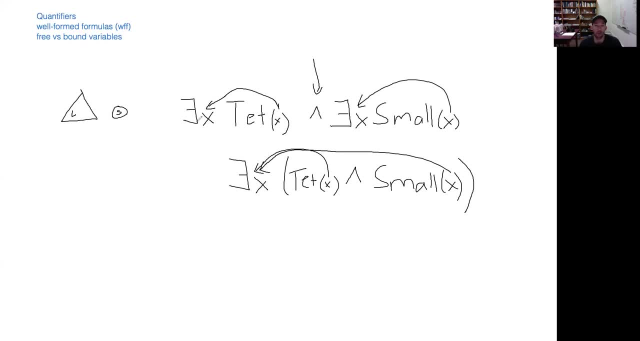 existential quantifier up front. So if I'm looking at a ruin, So say if I'm going to modify this next definition蛋. So, unlike above, where we had two instances of an existential quantifier and the different instances of the variables were bound by the two different instances of the existential quantifier, In the 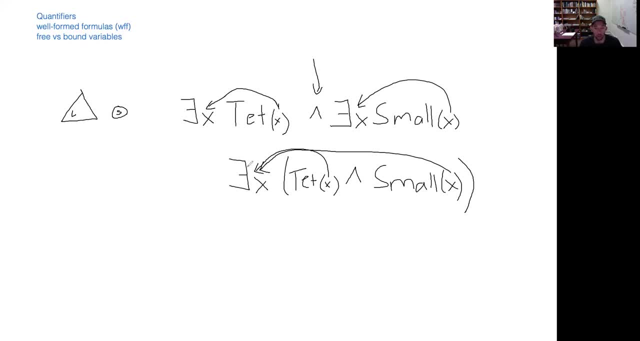 second sentence: we have a single existential quantifier and that's binding both of these instances of x, and we make that clear by realizing that, oh, we have here an open parenthesis- and this quantifier, the existential quantifier, ranges over all the instances of x that are within. 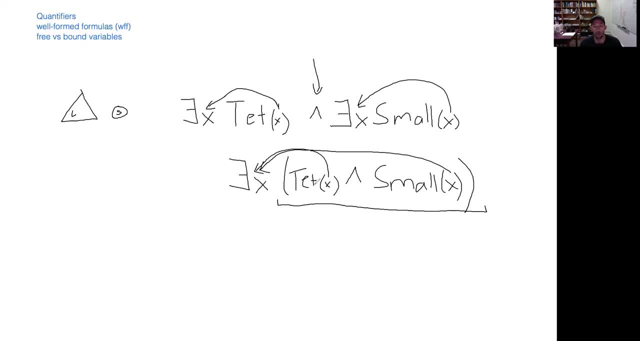 the scope of this parenthesis. So the scope of this existential quantifier ends right here. and then we've got and, and then this existential quantifier. it binds all the variables up to that point. Here we've used the the, this open parenthesis, to indicate that this existential quantifier 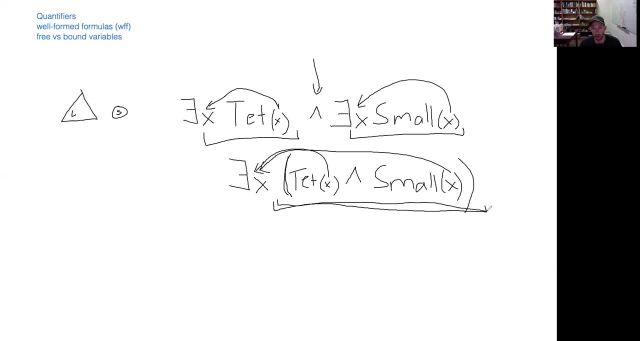 out front is actually binding, all the instances of x that occur inside those parentheses And this sentence will actually mean something very different. right, We're saying there there is at least one object that is both a tetrahedron and is small. So this second sentence maybe I'll. 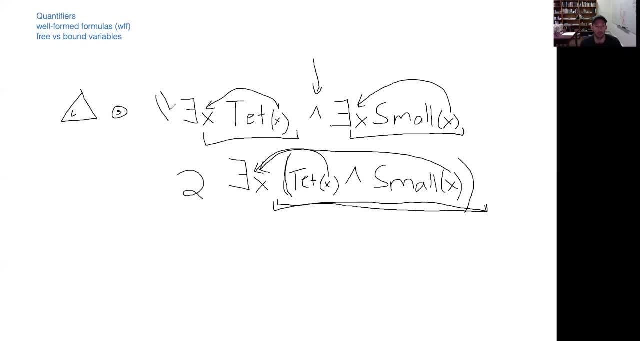 call this sentence one and I'll call this sentence two. Sentence two is going to be false in the world that we just developed. to make sentence one true, That's a terrible looking one. For sentence two to be true, what we need is a tetrahedron. 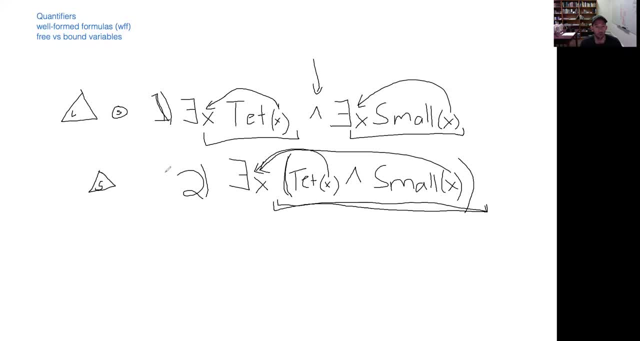 that is small. So two is made true in a world where there's at least one tetrahedron. that's small. Yes, this is the switch that I'm standing in. I'm standing in the middle of here. That's the edge. 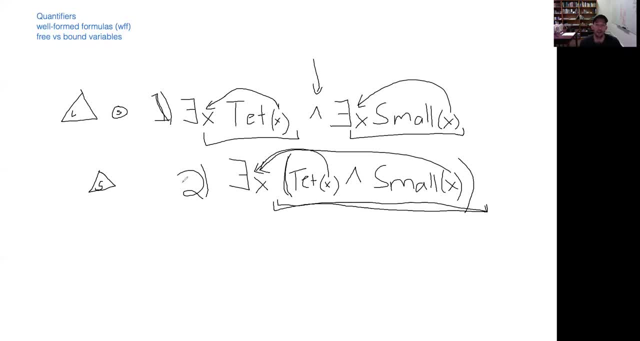 So the sentence has actually come to mean very different things, and the only difference is to note the ways in which we have bound the, the instances of the variable X. okay, so sometimes this will make a difference in terms of how to make. the sentence is true, and sometimes 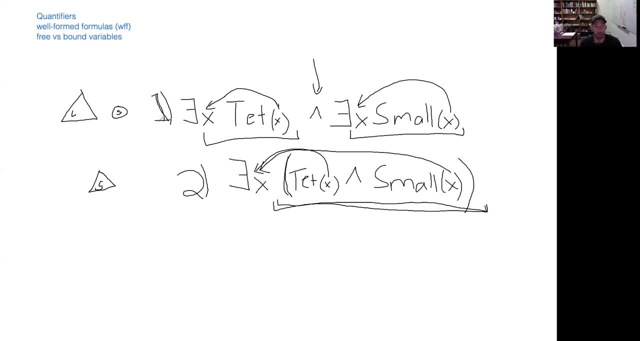 it won't. so, for example, right one and two have different meanings, and one of the way we can show that they've got different meanings is that there's a way to make one true but make two false. right, this world right over here makes one true but two false. sometimes, however, the sentences will will mean different. 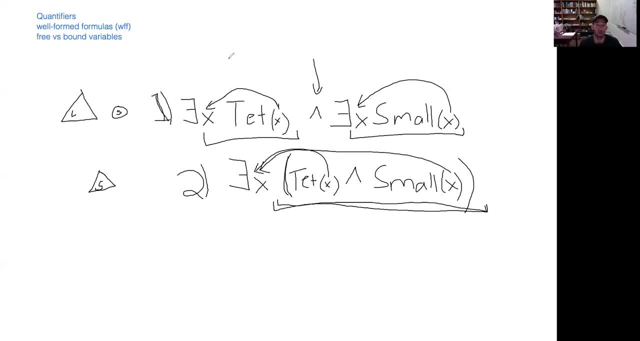 things but actually come really close to to finding or will come really close to being true in the same worlds. so here's what I have in mind. let's say, instead of having an existential quantifier out front in these two sentences, let's say instead that I put a universal quantifier up. 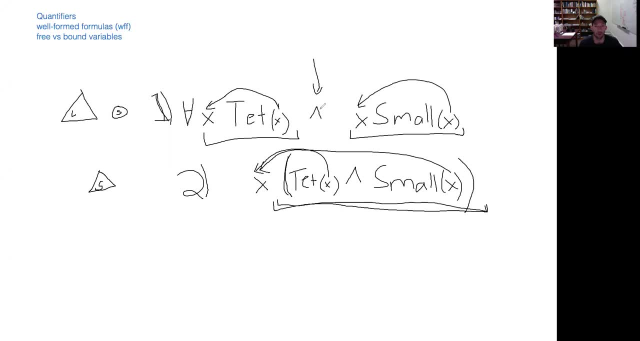 front, and now I want to compare these two sentences. the same thing applies it with respect to binding, that's to say, this instance of X is being bound by that particular universal quantifier, and this instance of X is being bound by that universal quantifier here, right in the, in this. 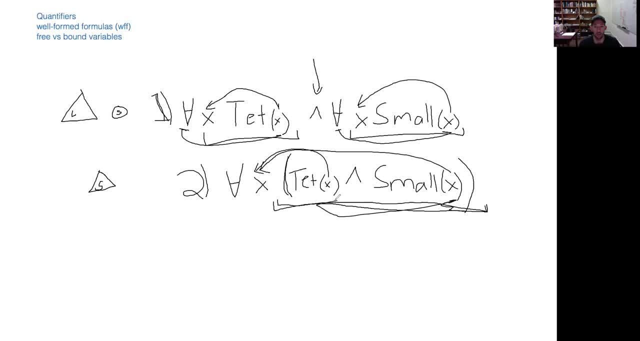 bottom case. again, we have both of these instances. this X and this X are both being bound by that universal quantifier. so what sentence one is saying, and when we use the universal quantifier, is that everything is a tetrahedron and everything is small and 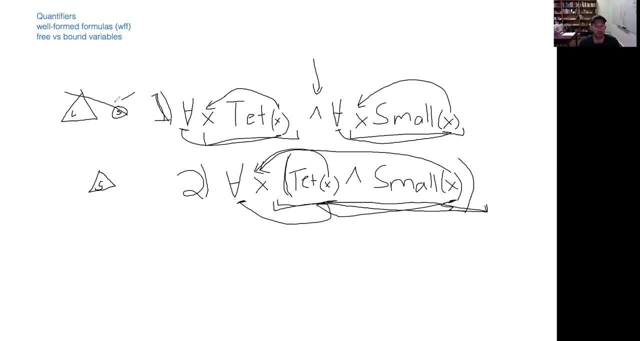 in. it's true while I'm using that expression, for each of the object is going to be as to be true or wrong. now notice that this world now would no longer be true. we'd have to have a bunch of tetrahedra, and each of them would have to be small ones. so one is made true, so long as.